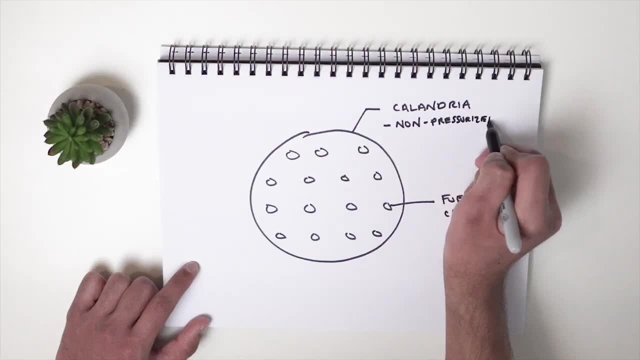 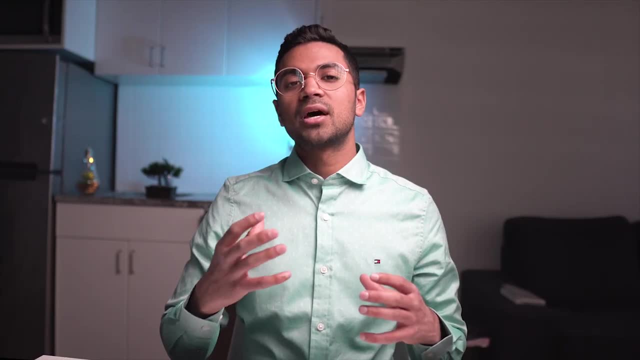 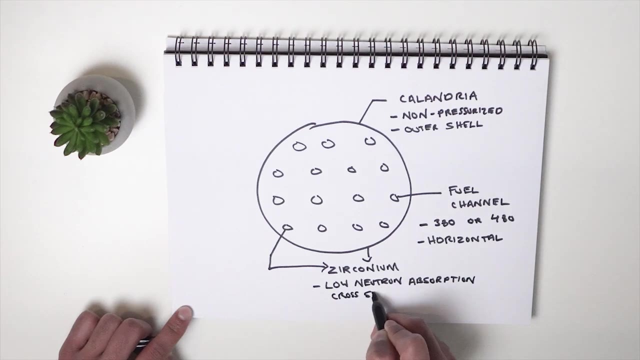 depending on the reactor energy capacity. Okay, so these fuel channels are horizontal channels which are made out of zirconium alloy. Zirconium is a metal which is unique to the nuclear industry because it's invisible to neutrons and also because of its capabilities of being durable and heat resistant. Many 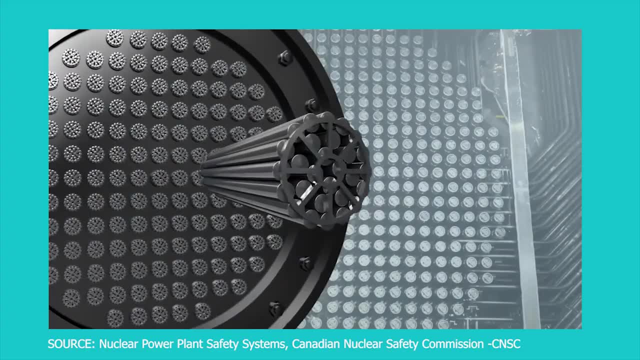 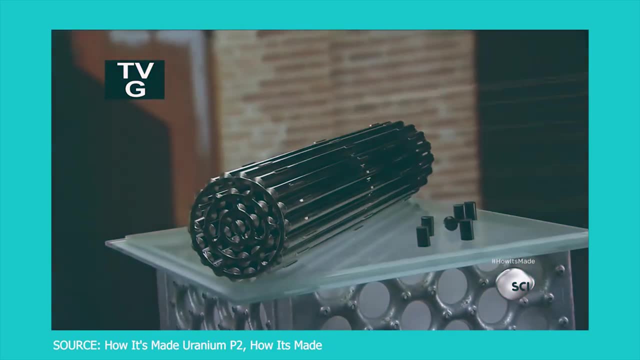 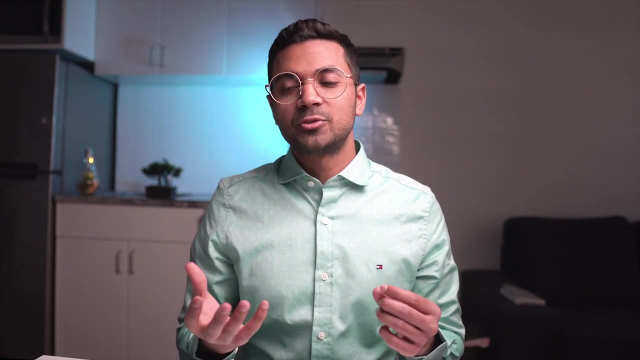 other properties which can be discussed in another five-minute video. These fuel channels hold pressure tubes which house fuel bundles. Next are the fuel, The fuel bundles. Fuel bundles are literally the size of a wooden log. You can hold the. you can hold a fresh bundle safely in your hands. The reason why is because the 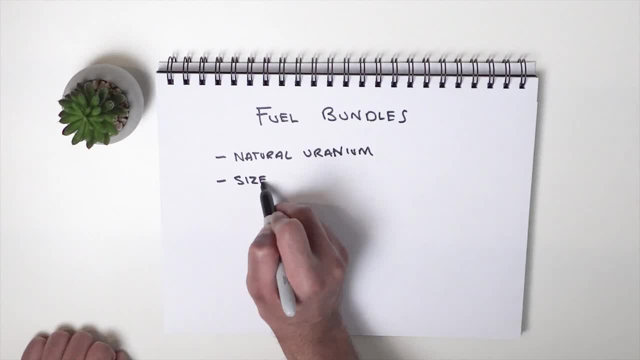 fuel is made out of natural uranium, so it's mined from the ground. It's literally a rock which is processed and stored in the ground. It's made out of natural uranium, so it's mined from the ground. It's literally a rock which is processed. 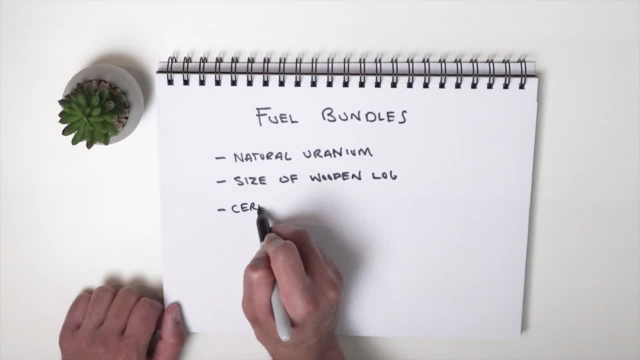 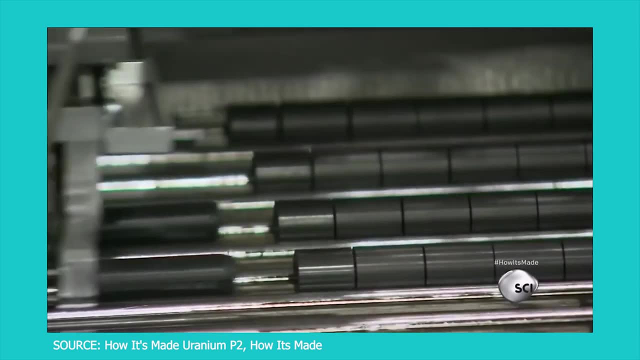 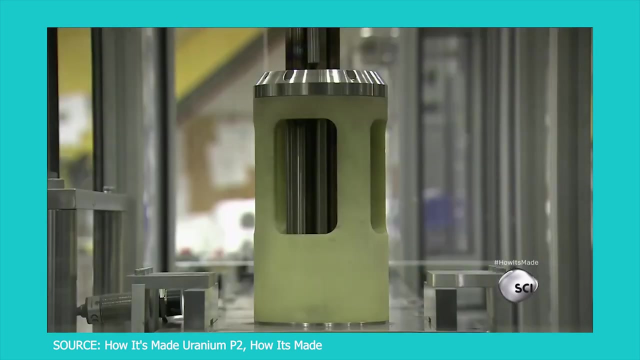 into fuel pellets. These are ceramic fuel pellets. Ceramic because ceramics are really good. They're heat resistant and these pellets are housed in these metal sheaths. okay, or the bundle itself. CANDU is unique because it also uses natural uranium instead of enriched uranium. Now what's the difference between the two? 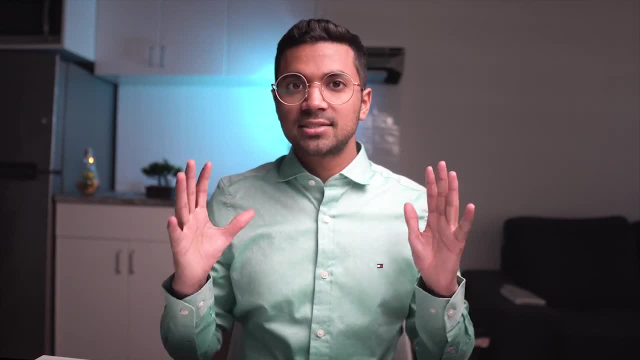 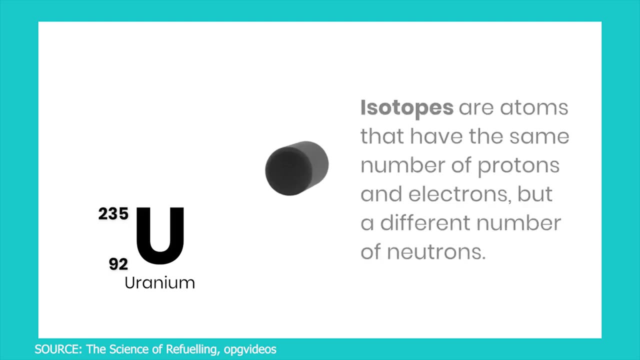 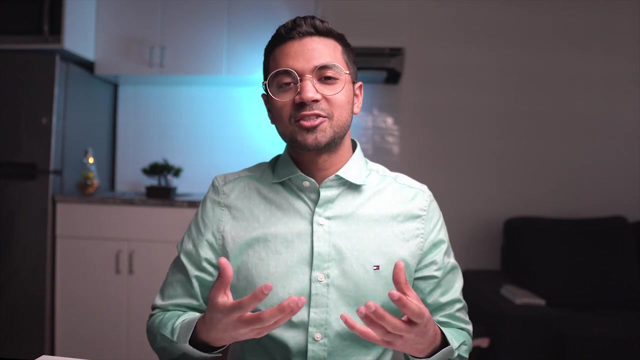 Higher fission content. Okay, so uranium that exists in nature has an isotope called U235, which is very less in nature. Now, coincidentally, this isotope is what actually does all the legwork when it comes to fission. It's what helps produce the fission reaction, which, in 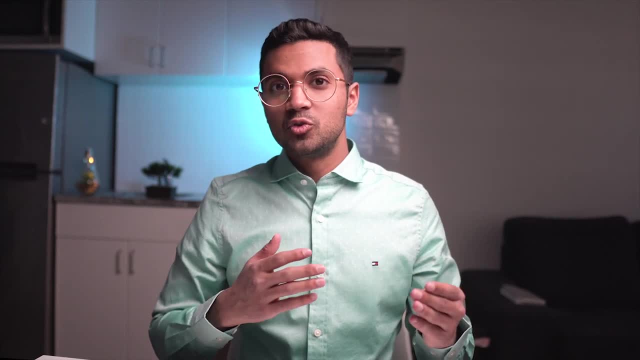 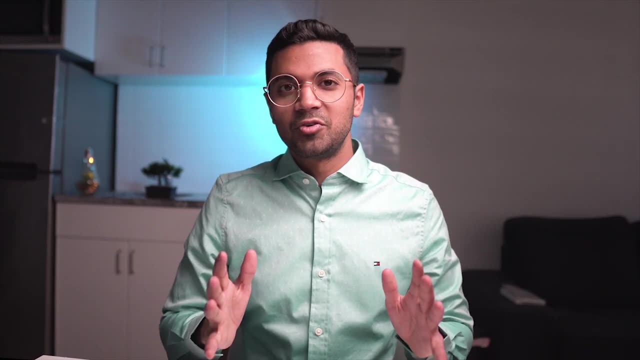 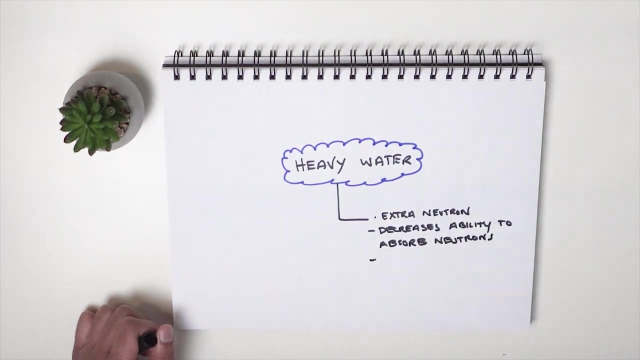 turn, produces heat. Now, to mitigate that, the CANDU is unique because it uses heavy water instead of regular water. So let me simplify the physics behind heavy water. Now, heavy water has an extra neutron, which decreases its ability to absorb excess neutrons. Now, since heavy water doesn't absorb as many neutrons as 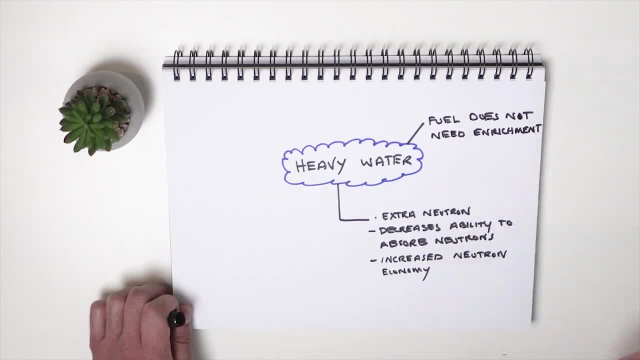 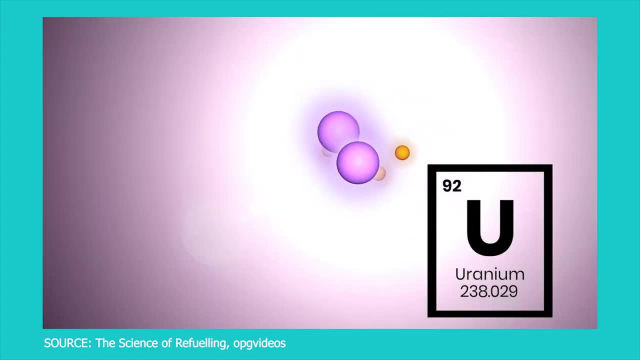 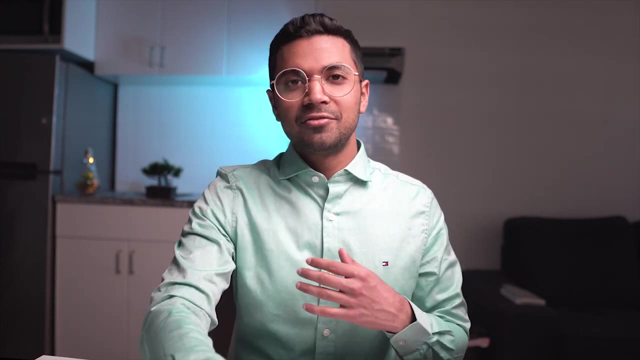 regular water. it provides better neutron economy. Now, why are we talking about neutrons? Well, neutrons are what start the nuclear fission reaction. So more neutrons, better neutron economy means more power output, and you don't necessarily need enriched fuels. What are the advantages of using natural uranium? 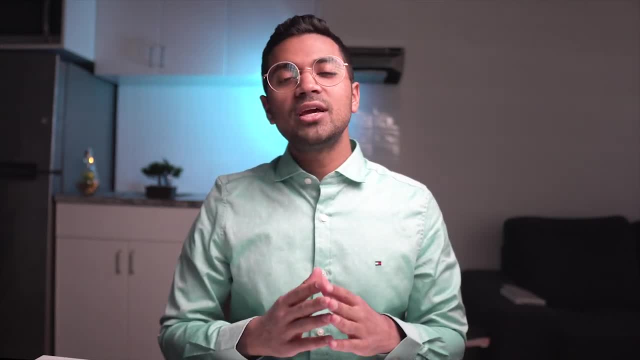 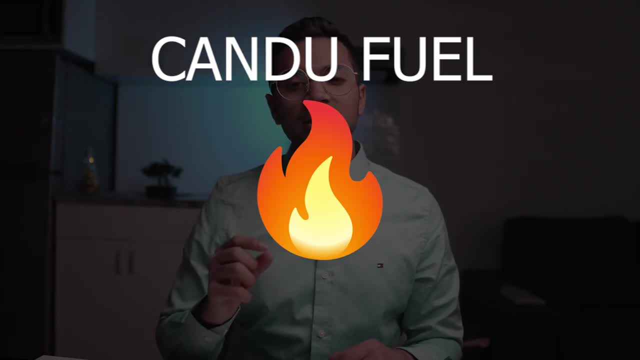 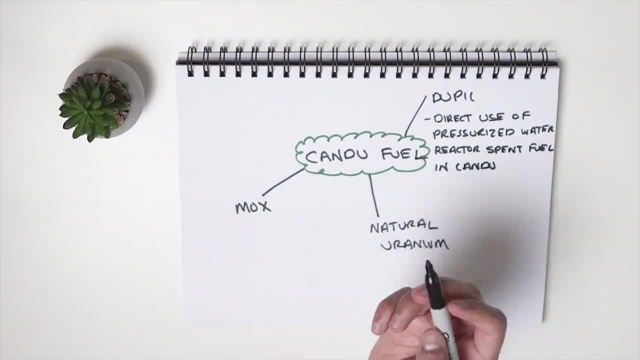 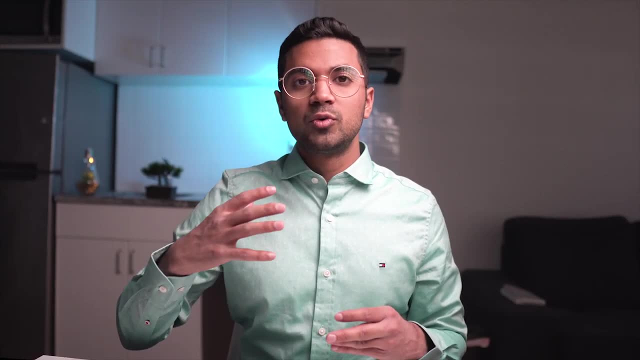 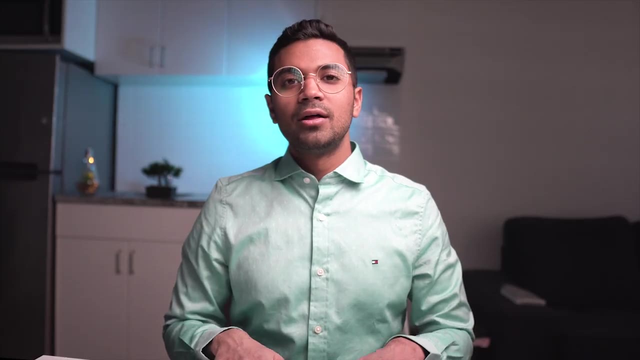 reprocessed and used in CANDU. It can also use mixed oxide fuel, MOX, which is another type of recycled fuel. also, it can- it can- use future fuel sources like thorium. Now let's go into on-power fueling. What is on-power fueling? Well, imagine filling up your car while it. 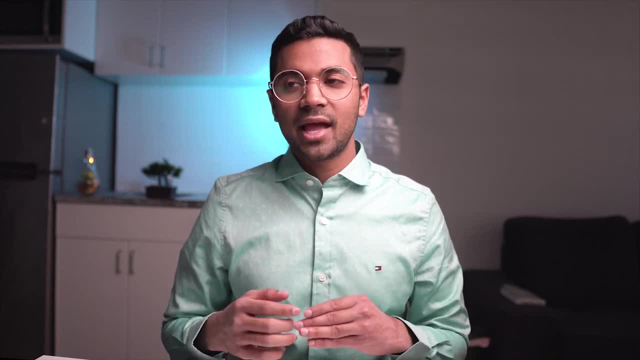 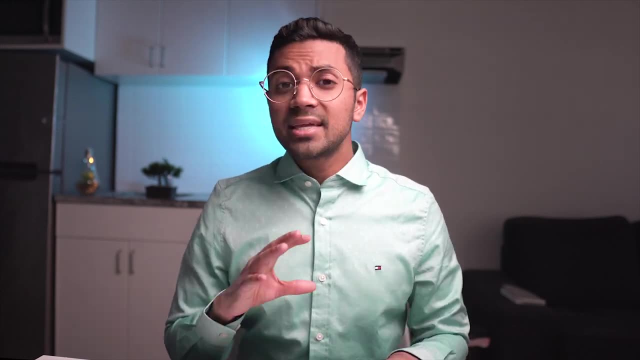 while it's running, and it's running 24 seven. Well, this is what a CANDU can do, but safely. Now, conventional reactors, they need to be shut down for months at a time to replace fuel. CANDU is unique because it can have its fuel replaced. 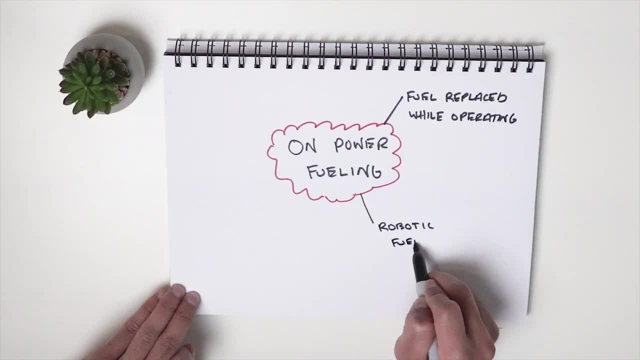 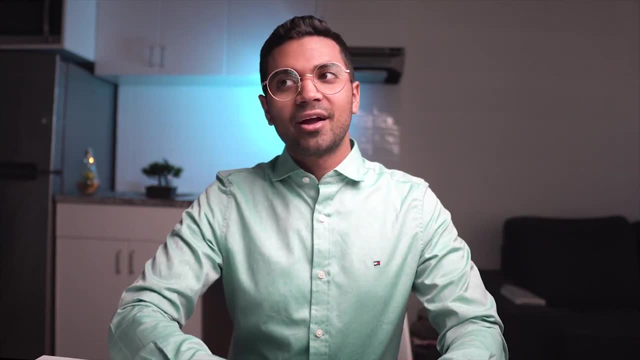 while it's operating okay. So CANDU reactors are equipped with robotic fueling machines which can pump in fresh fuel and take out used fuel. This is why CANDUs have a very high capacity factor, meaning the amount of days in a year. 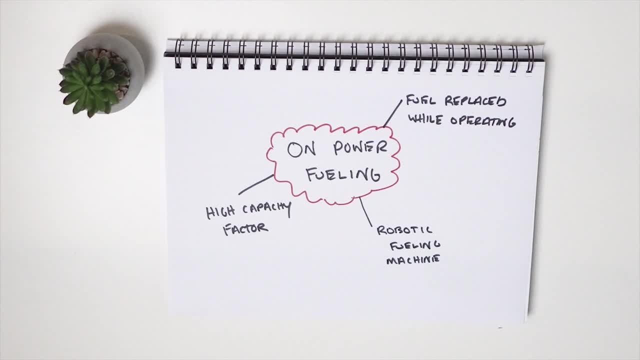 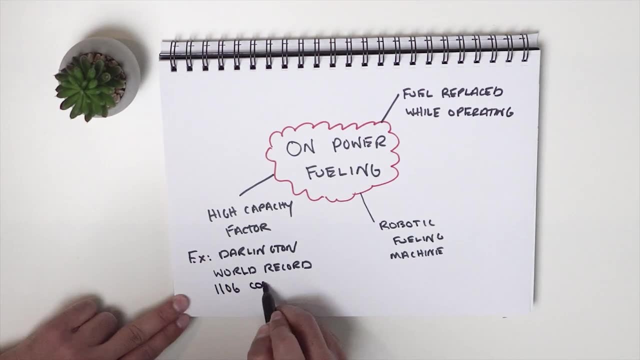 that the CANDU is operating is immense. These reactors can operate years on end before having to be shut down for maintenance, And the reason why is because of this unique feature on power fueling. Okay, so let's move into safety systems. 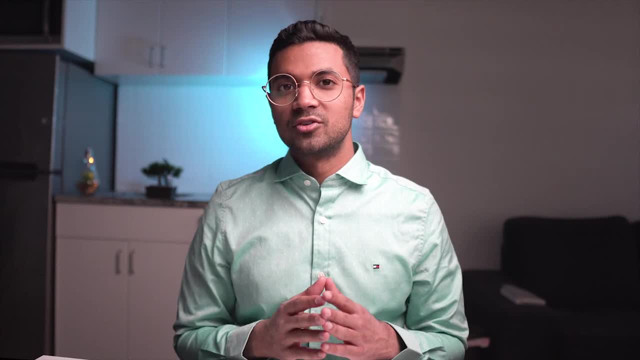 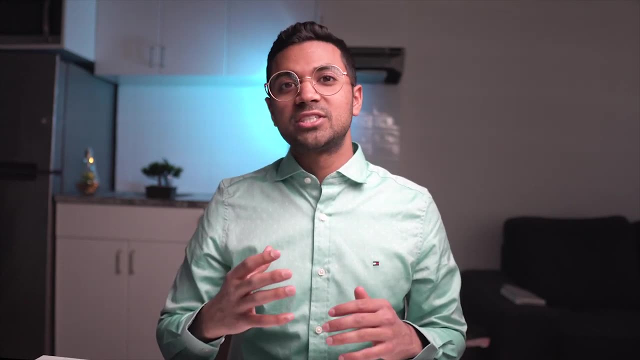 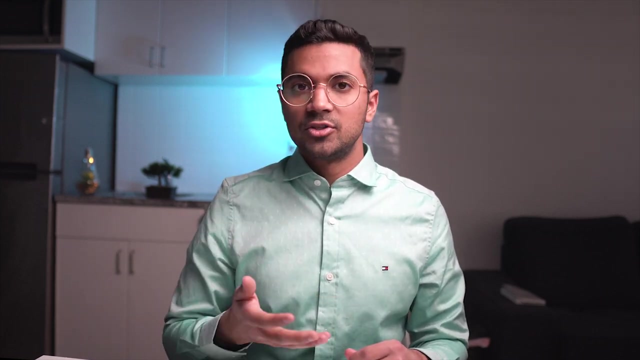 CANDU is one of the safest nuclear reactor designs. It's literally the Volvo of nuclear reactor. I could do a two hour video on just how safe this reactor is and its safety features, But in the light of this five minute video I'll just be going through the top kind of safety features. 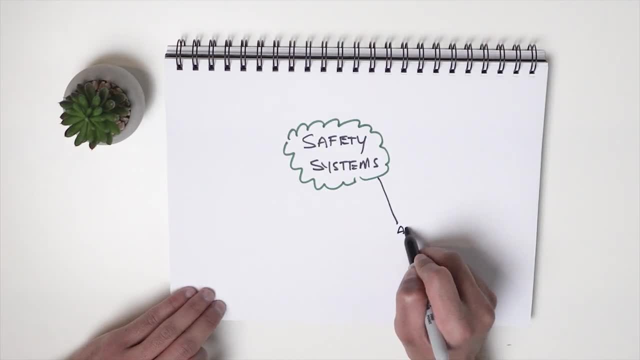 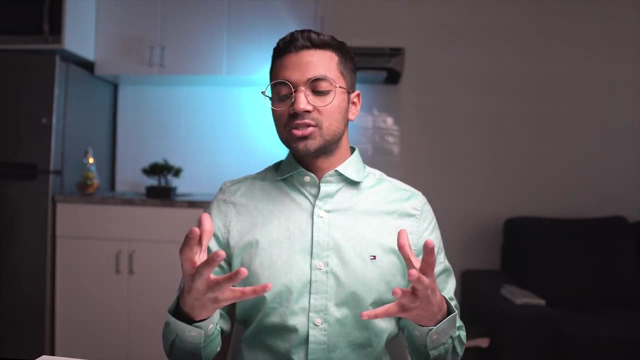 that this reactor has Number one adjuster rods or control rods, which is the primary shutdown mechanism. So these rods are made out of a metal called cadmium, which is an absorber of neutrons. Once rods are injected into the system, 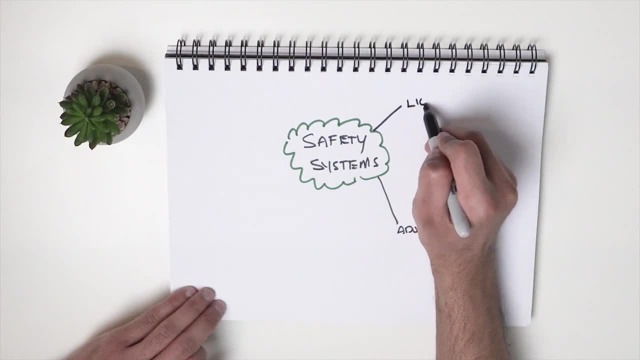 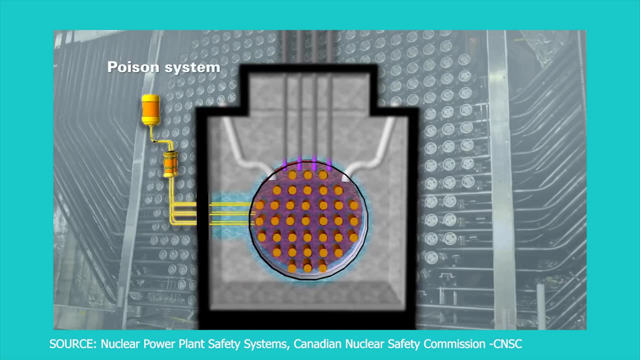 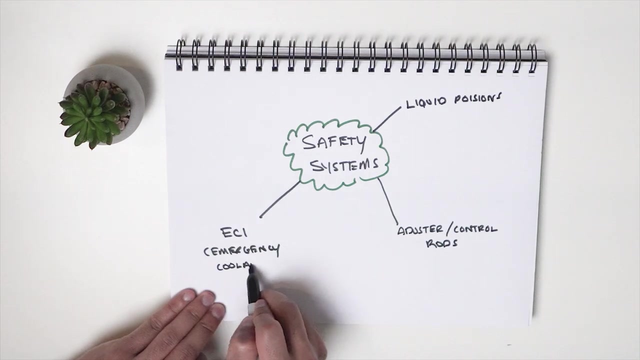 it's shut down within seconds. Number two is injection of a chemical liquid or a called a poison. So these poisons called gadolinium nitrate pushed into the reactor and can also shut down the reaction. Number three is ECI. Now, ECI is used when there's a loss of coolant.